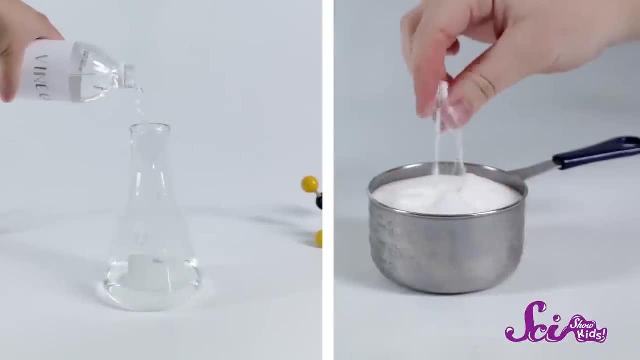 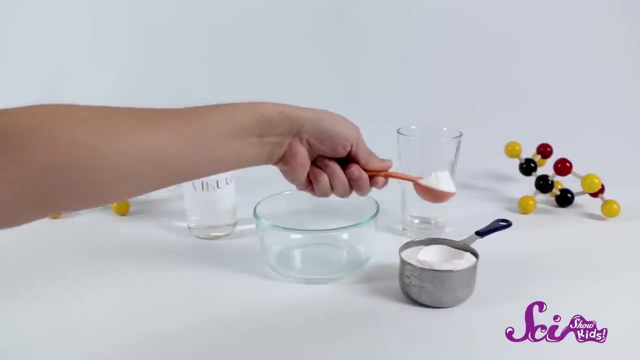 Is it a solid? No, it's a liquid, And both of these things stay that way, Unless you mix them together. Let's take a look. First take one big tablespoon of baking soda and put it in the bowl, Then measure out six tablespoons of vinegar and put it in the glass. 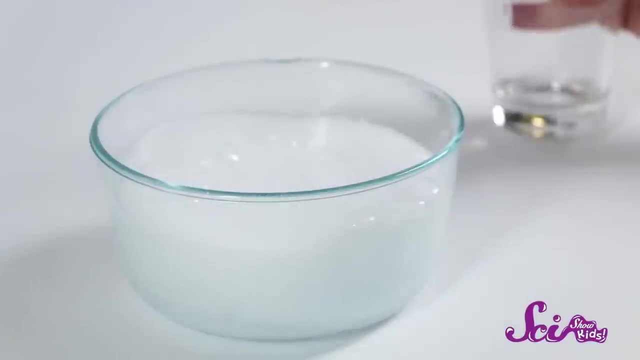 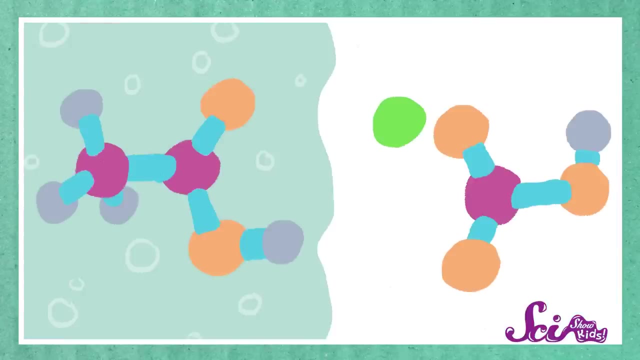 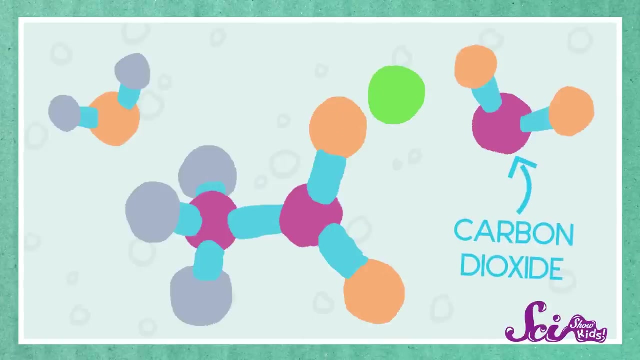 Now slowly pour the vinegar onto the baking soda. Awesome. When the baking soda and vinegar mix together in a reaction, the tiny parts that make up the chemicals rearrange themselves and they make something new. Those bubbles, you see, are carbon dioxide, which is a gas. 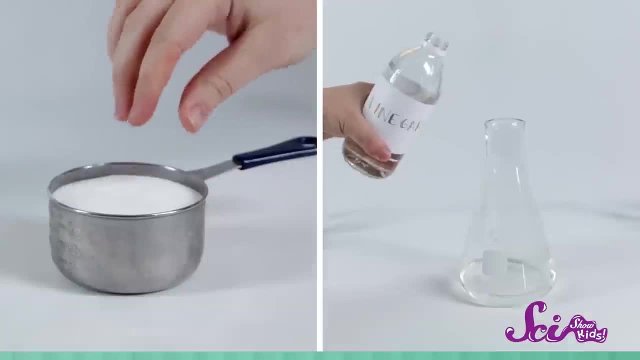 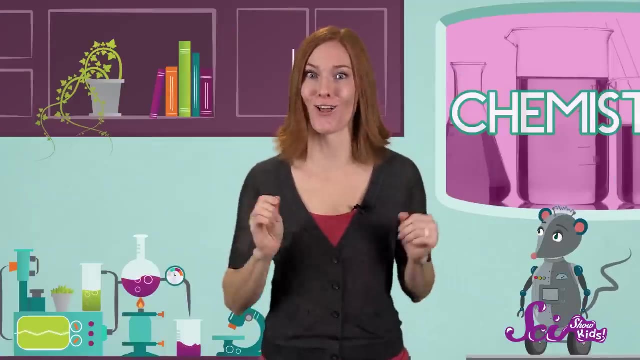 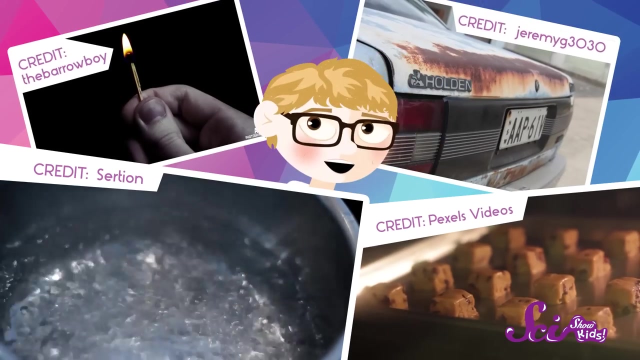 It's the same stuff you find in bubbly drinks. So when the solid and the liquid came together, they made a gas. Chemists study all kinds of reactions a lot like this one, And since everything is made of chemicals, that means there are reactions going on all around us all the time. 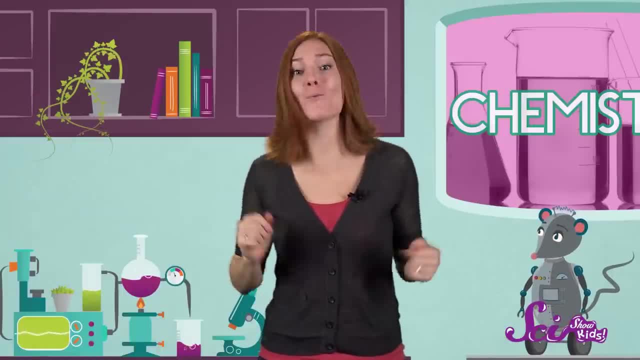 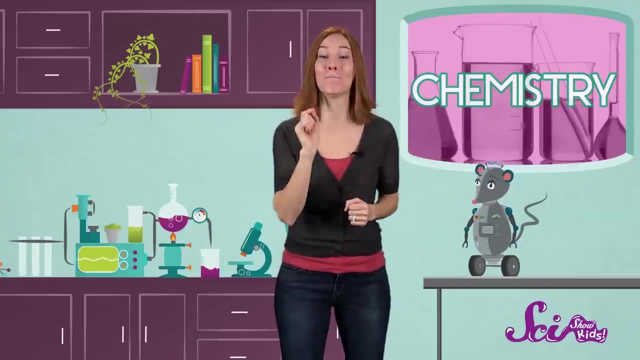 Chemists know how to control the reactions to get the things that we want and need. Like what? Well, some chemists study how chemicals work in the human body. That's right, Your body is made of chemicals too, And these kinds of chemists might work to make the perfect medicine to fix a tummy ache. 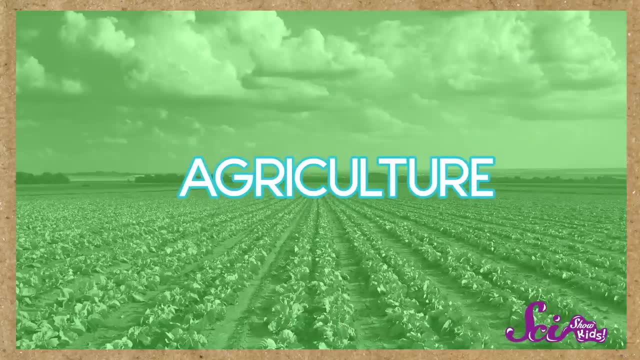 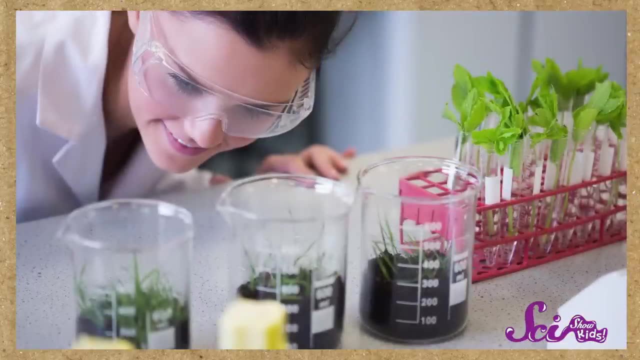 or a better shampoo to get your hair clean. Other chemists look at how chemicals interact in the environment. They may make products that help farmers with their crops or help figure out what's in the soil or water. Some chemists work with non-living things. 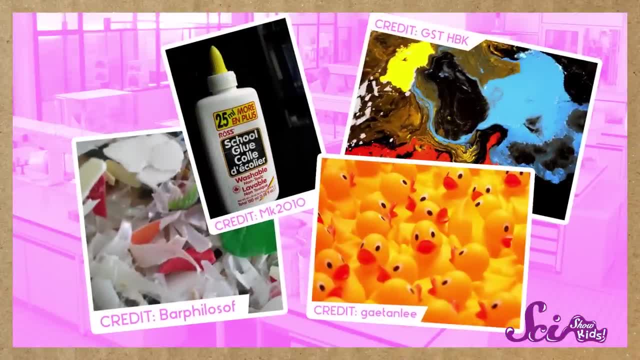 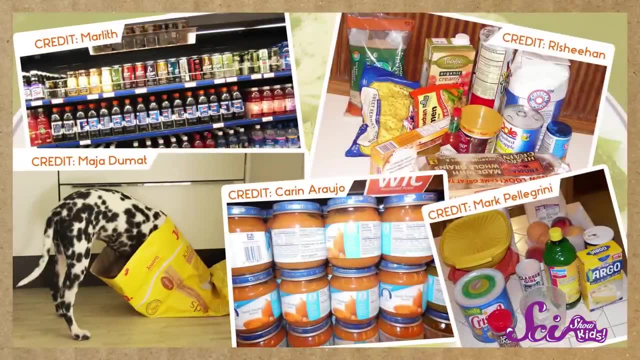 learning more about things like plastic, paint, glue and rubber. And then lots of other chemists work with food, Drinks, packaged food, pet food, Baby food, Baking ingredients. Chemists work with all of these things to make them tasty and safe. 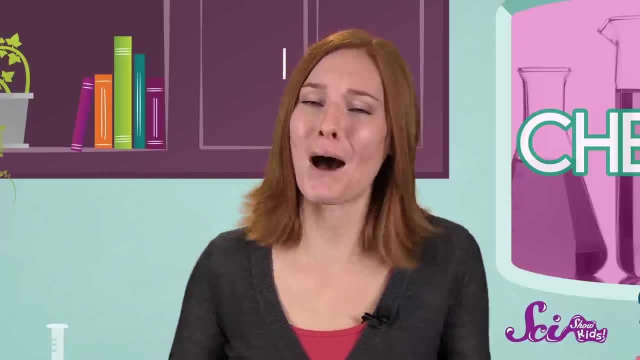 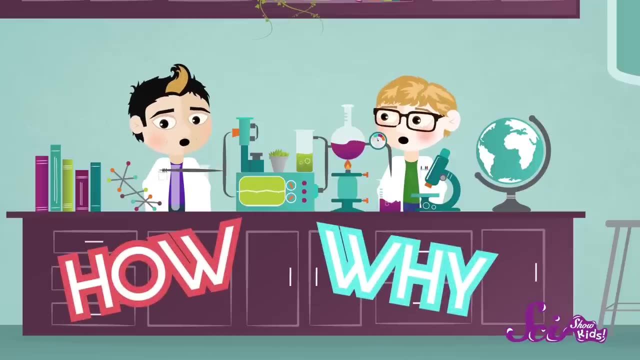 All kinds of stuff that you use every day is possible because of chemists. Being a chemist is super cool. You can learn how and why things happen to all the stuff around you, Not to mention you get to mix things up, make a mess. 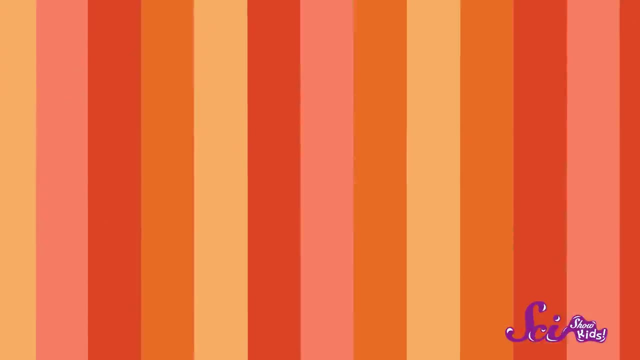 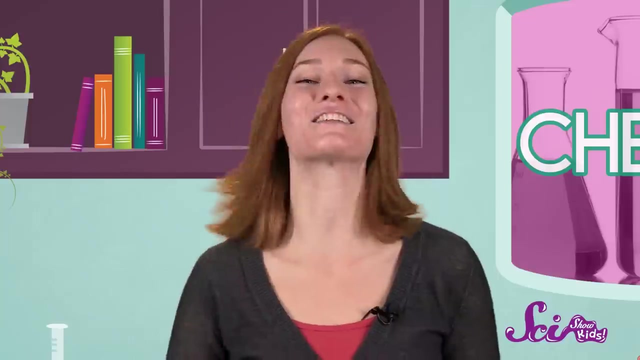 and watch wild and crazy reactions. So do you think you might want to be a chemist? Stay curious about all the stuff around you and pay close attention to how it changes, And you can start right now. Did you try our experiment with baking soda and vinegar?